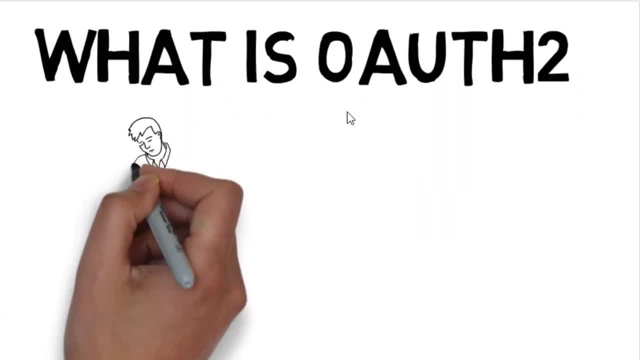 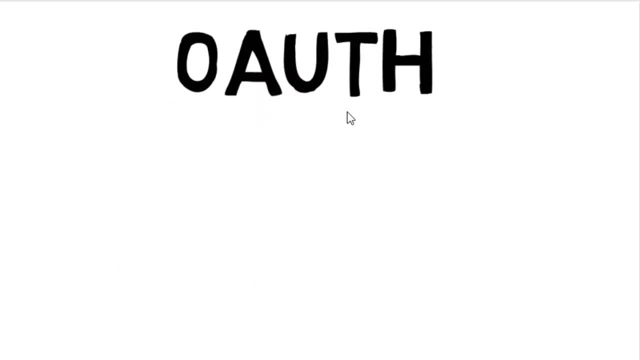 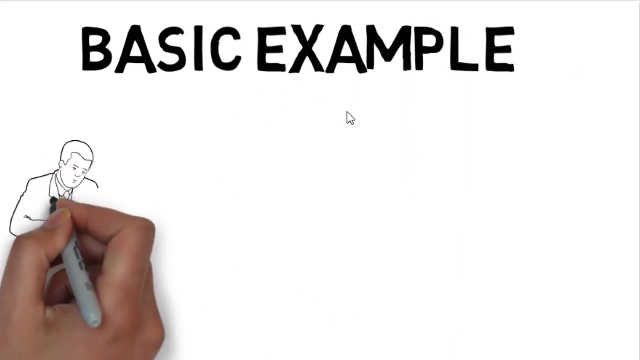 Welcome friends. My name is Gautam, So in this tutorial we will be talking about a very famous authentication protocol known as OAuth2.. So it is used for authentication applications. So it stands for open authorization. So in this slide you can see that it stands for open authorization and it's kind of a protocol. And let me take a very basic example in order to illustrate to this protocol. Let's suppose we have a client and we have a server. So this is a client. 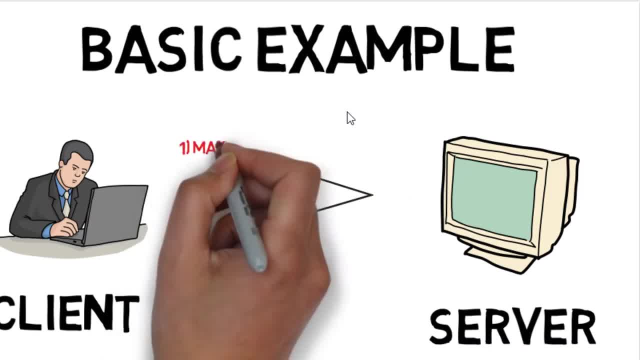 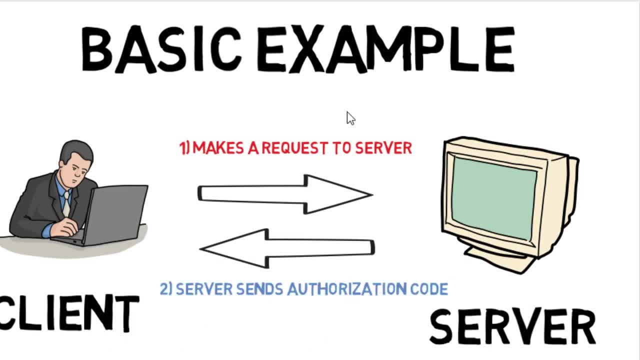 And this is a server And let's suppose a client makes a request to the server And then the server just sends back the authorization code And then the client uses that authorization code and sends that code to the server And then the server returns the access token. So with the help of this access token the user can access the API, can request the profile information of the user. So this is kind of a very basic example. So let me talk about some of the terminologies. 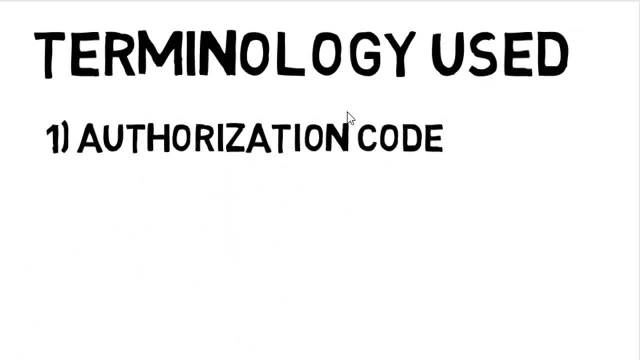 that is used in the previous slide. First is the authorization code, So we will discuss about all these things. And second comes is the scope- Scope is kind of what information your app is requesting from the user. And third comes is the redirect URL, a specific URL that is assigned by the server. And fourth is the access token, with the help of which you can request information about the API or request user information. So, basically, first of all, let me talk about the authorization code. 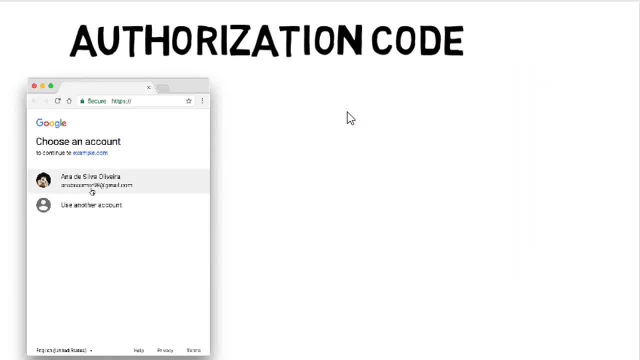 So basically authorization code. you can see in the example here also a list of accounts is there of the particular user. You select particular account And then after that, with the help of this authorization code, you allow certain information scopes. You can see that in this it is requesting some scope information. So it is the first step which comes in OR2.. And in this step you can see that the user grant access token. 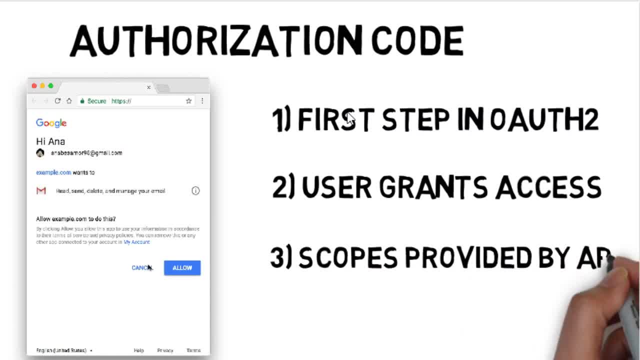 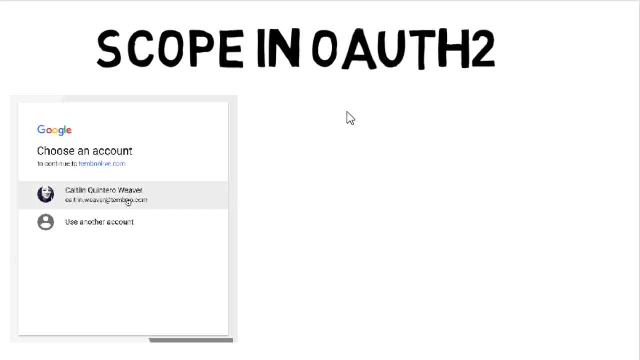 So you can see that the user grant access to certain kind of scopes which are available. So scopes are nothing but what kind of information your app is exchanging for the user. And then this authorization code is exchanged for access token. The access token is granted by the server to the application. So this is all about the authorization code. So next come is the scope in OR2.. So basically, as I told you earlier, scope is kind of the information that the app just 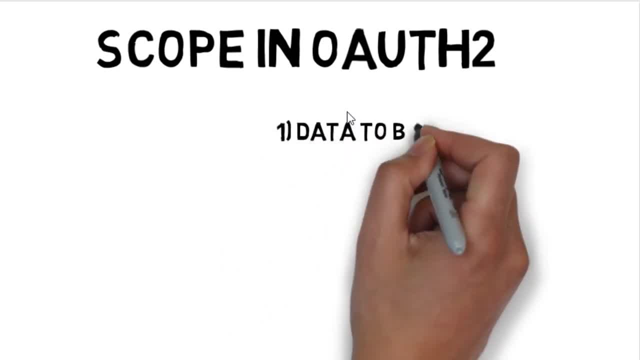 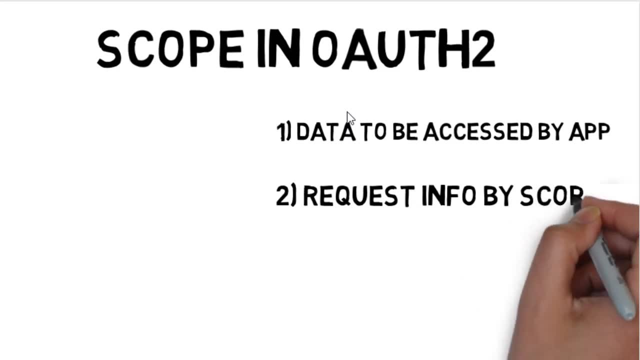 gives you. It records all information about the application. So, basically, it provides the scope of the application and it can generate data in form of a specific scope, which is a pretty big if you search for six scope, script tasks and scopes. So basically, let's go ahead and let's look at the code in the application. SO basically, let's. 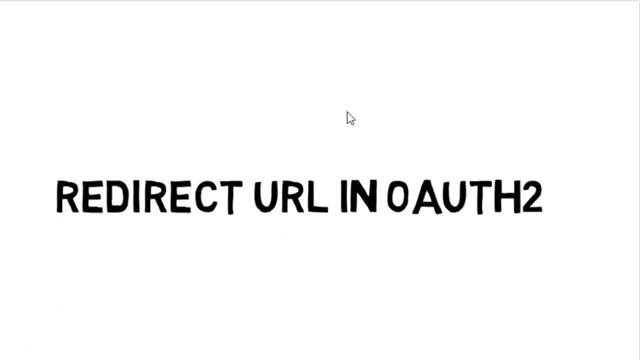 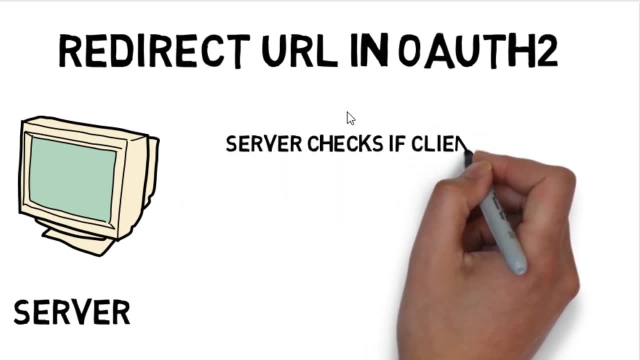 see what these scopes will be, which are the scopes that all of the data in theppe application that we are going to look at today. So let's go ahead and let's quickly go ahead and explain this first step. So it, George, George, so X. 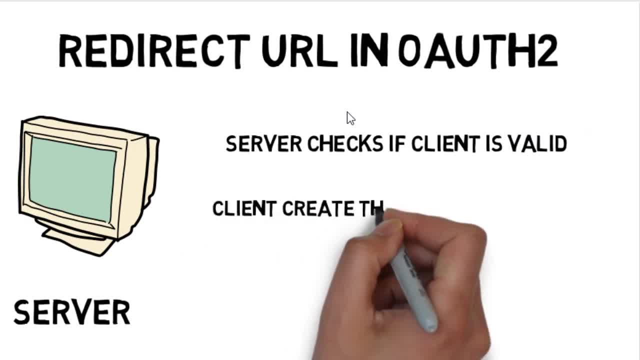 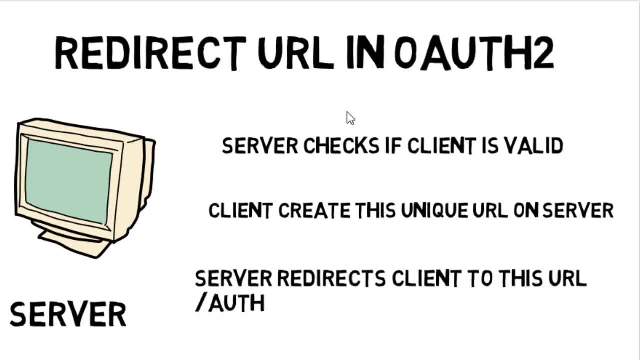 It is useful for checking if the client or if the application is valid or not, and this URL is generated on the server side and then the server redirects the user to this URL. Let's suppose: slash auth, slash client auth, You can just create this URL. 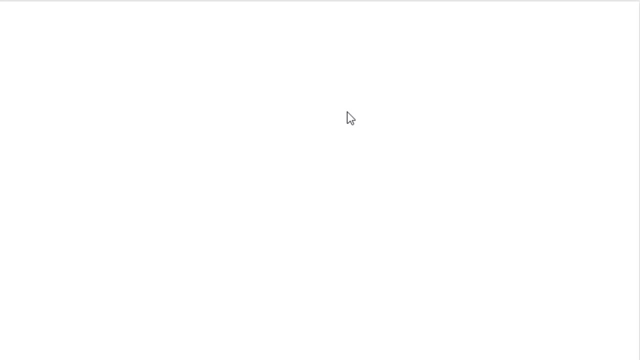 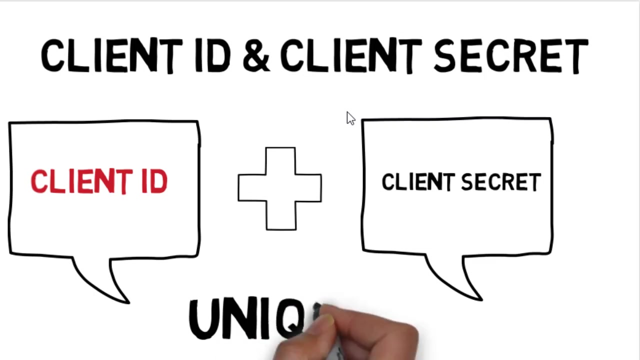 So, basically, this is all about the redirect URL. Now comes the client ID and the client secret. So this is part of the information that you have to set up before you can make your OAuth 2.0 application. These are two unique information that you want to store anywhere. This is client ID and client secret. 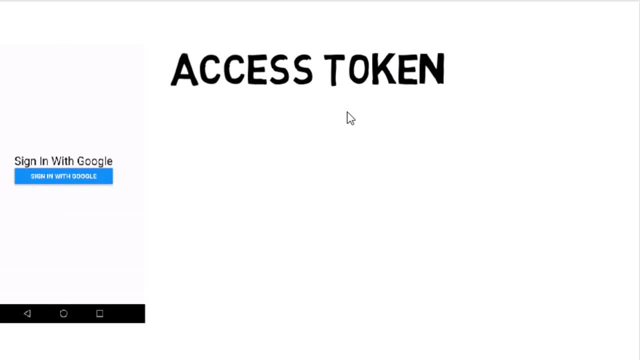 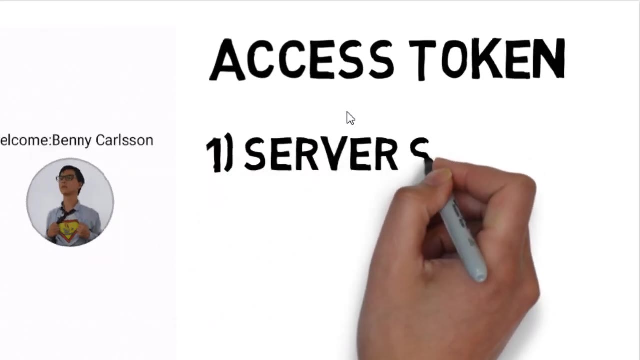 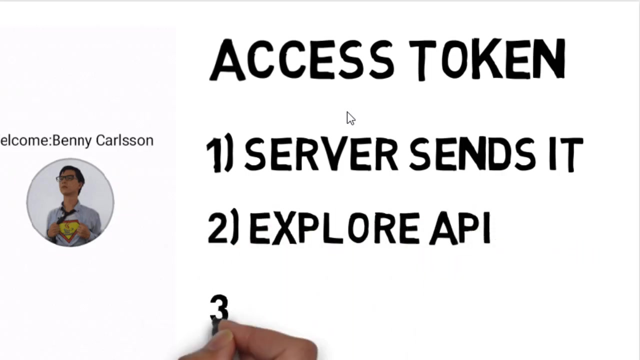 And, last but not least, we have the access token. So, as I told you earlier that with the help of this access token, we can make your OAuth 2.0 application, So with the access token, which is generated by the server, you can request API, you can request profile information. In this slide also, you can see that it is requesting the profile information, that is displaying the profile picture, and the server sends it. This is the very most important thing and with the help of it, you can explore the API or you can request the profile information or user data, in this case, the display picture. you can see that You can also request email ID, date of birth, etc. All these things.